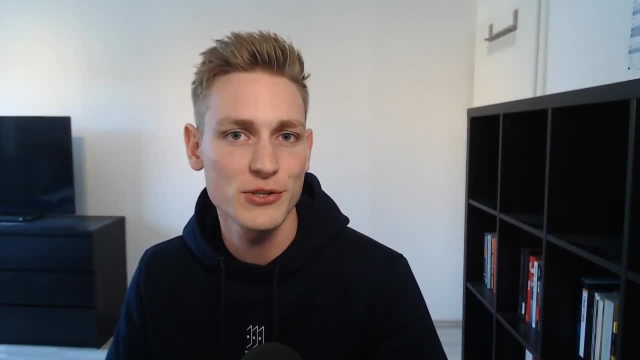 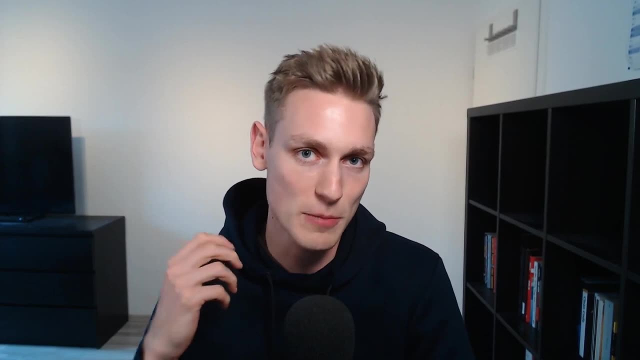 So what is Shopify's API? why is it important and should you be using it too? Let's find out together. Hey everyone, Jan here. Welcome back to Coding with Jan. Today we will get started with Shopify's API. We will take a closer look at what an API actually is and what they are all about, and then 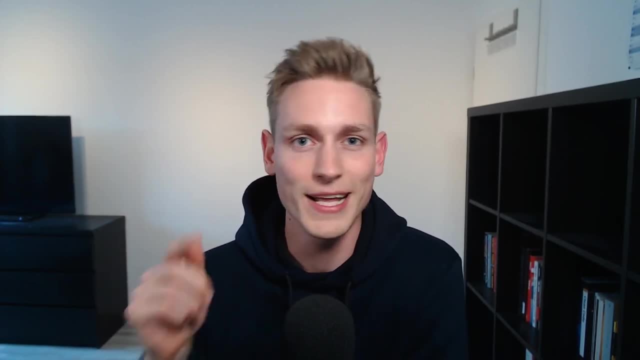 I also have some practical or real world use cases and examples for you and some tips on how to get started. These days, it feels a bit like everyone is talking about APIs and it's not like everyone- everyone- but at some point you may come across someone who is actually talking about an API. 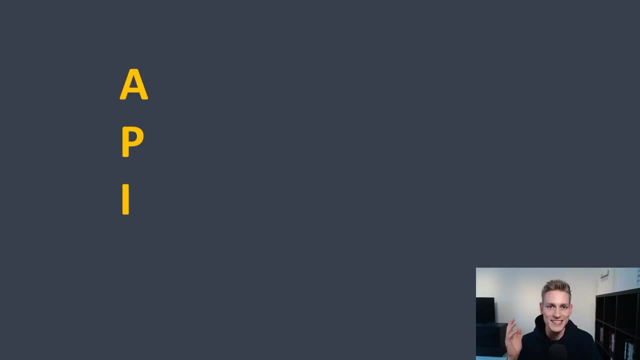 and then you will be prepared, So let's dive right in. Alright, so let's get started with what an API actually is. The term stands for Application Programming Interface, and as this doesn't really explain anything, I have prepared for you a very common and intuitive analogy. So let's imagine: 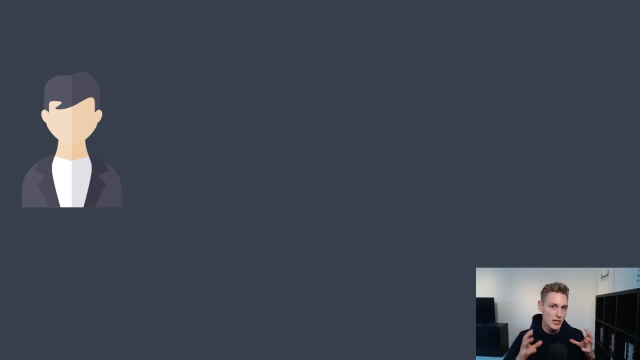 that you're going to a restaurant and the restaurant itself is actually a quite complex system if you think about it. So, for instance, you need a cook who knows all the different recipes. then you would also need some information, infrastructure and kitchen appliance and people that know how to operate these dishes need to be. 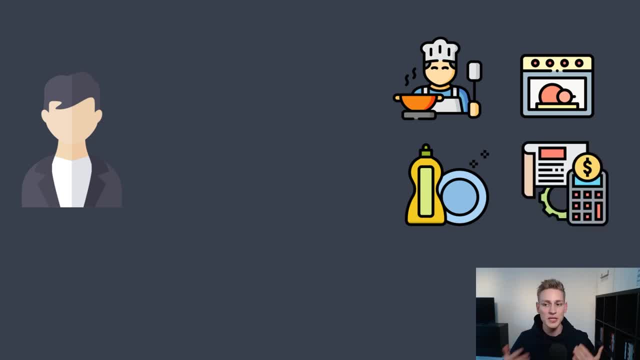 cleaned and managed in some way. and then you also need some order system and bookkeeping- all the things that no one wants to deal with. but the convenient thing for you as a guest is that you don't need to know anything about these things because we also have the waiter. 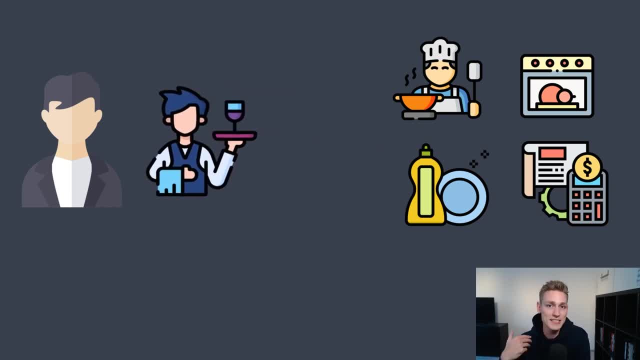 which is pretty much the only person you need to talk to, and you can ask him questions. you can ask him for drinks, he gets you the food, he gets you the bill and pretty much anything you want, without ever getting in touch with all the stuff behind the scenes. so one way. 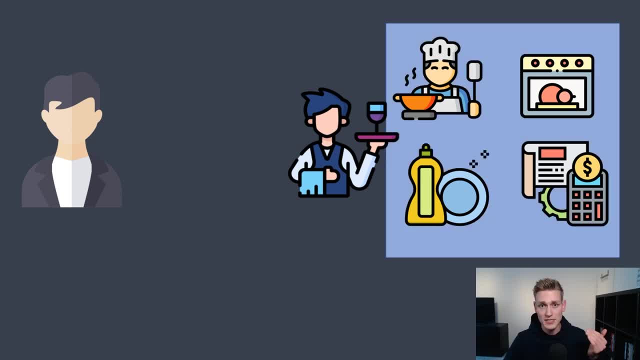 of thinking about this would be that the waiter actually shields you from all these processes, and then he represents the interface that enables you to communicate and interact with the restaurant system without ever knowing what happens in the background. So, in this particular case, the waiter can be seen as the api of that restaurant, because he helps us to communicate. 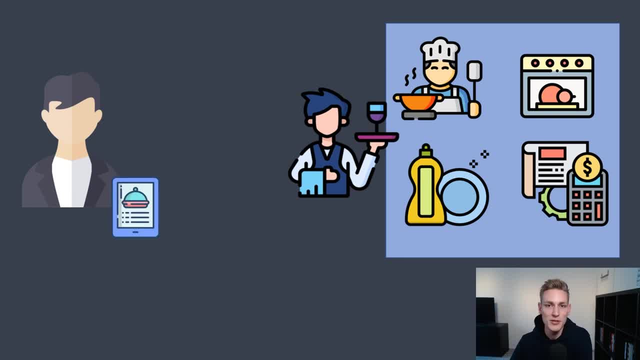 with the system behind him and, if you want, the food menu could be seen as the api documentation for food and drinks, because it tells us exactly what kind of food you want to eat and what kind of requests we can make, and it also tells us what you expect to get back, or in other words, 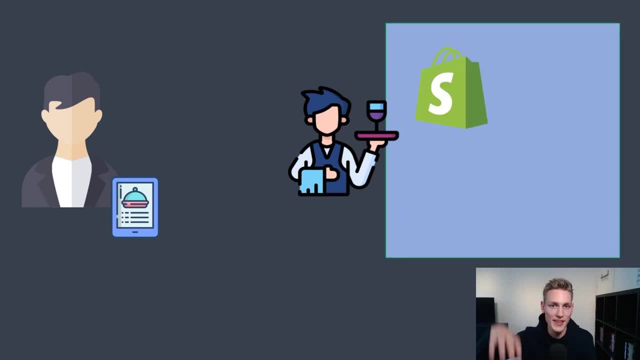 what the response might look like. and now we have to transfer that knowledge to the shopify space, and shopify is an at least equally complex system. we have no idea how databases look like exactly. we have no idea how exactly they save the products in there. we don't know how they handle charges. 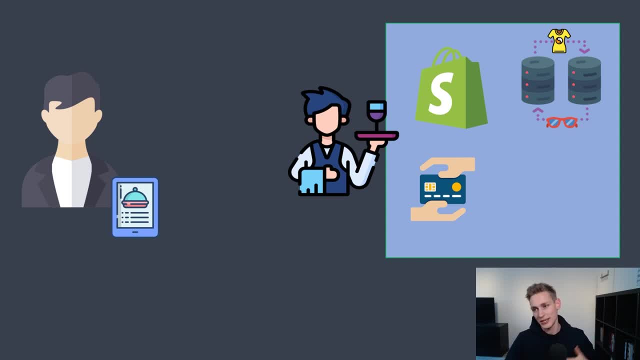 how they work with different banks and payment providers. we don't know how exactly the card system works or how the order system works, but we have to transfer that knowledge to the shopify space. The food menu turns into shopify's api documentation and the guest should look a bit more developerish. 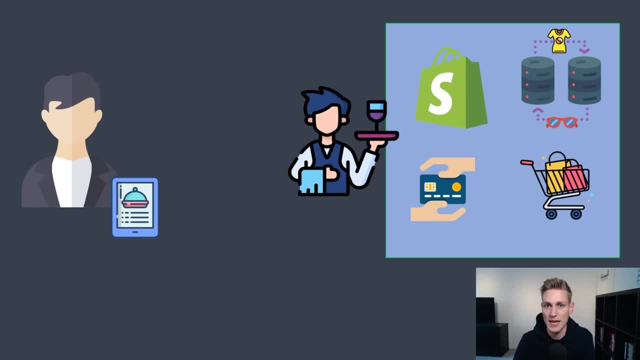 because we can make use of them just by communicating with the api. and now let's give it a little more abstract illustration. the food menu turns into shopify's api documentation and the guest should look a bit more developerish. then we add two dashed arrow lines to make. 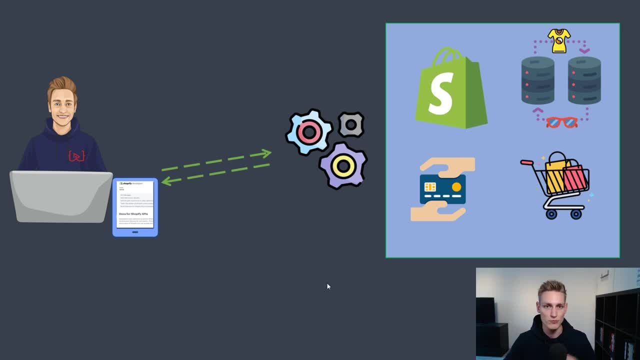 everything look scientific and voila. there you have it. so let's wrap everything up one more time. we have a complex system where we don't know exactly how everything works, but we know what the system offers because everything is well documented, and then we have an easy to use interface which allows: 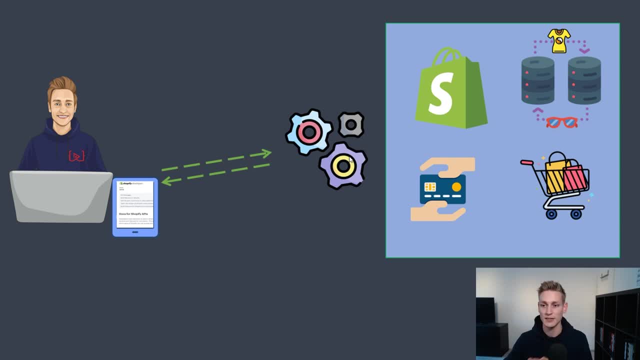 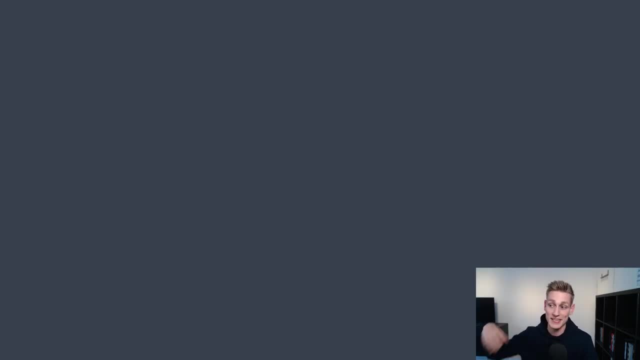 us to communicate with the system, exchange information and use the services it offers, and that's namely the api. all right, so now, before we get into the practical use cases and examples, i want you to know that shopify has like two main apis. one is called the admin api and one is called 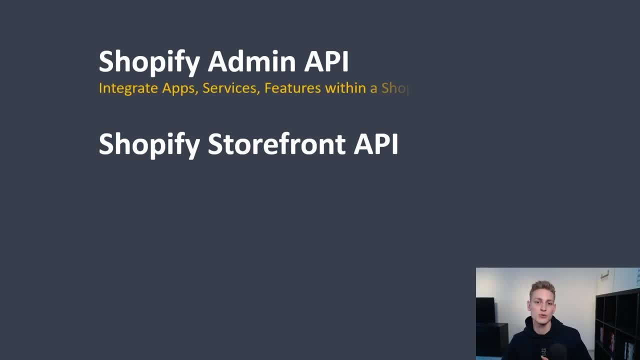 the storefront api, where the admin api is used to integrate apps, services and features within the storefront api. so, for example, this could be: you want to collect email addresses on your front page and you want to pass these email addresses to your third-party email marketing tool. then you would use the admin api and the storefront api, on the other hand, is used to 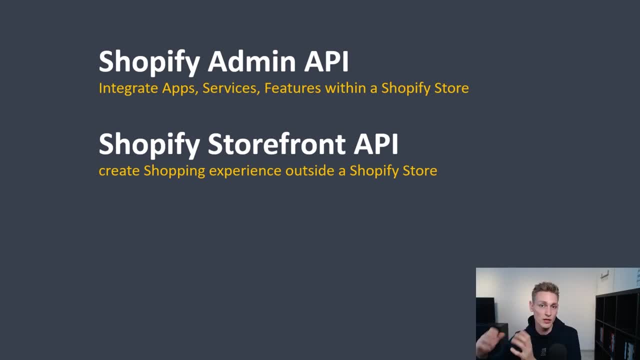 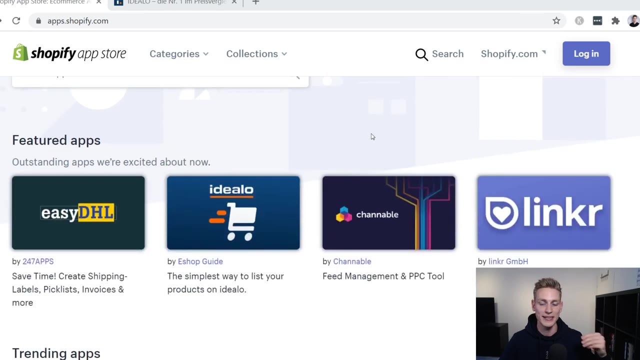 create shopping experiences outside a shopify store or apart from a shopify store, and this could be if you want to give customers the opportunity to buy products in different places than your online store or your theme. better to say, but i will show you what that means in a minute now as a first real world example. i actually want 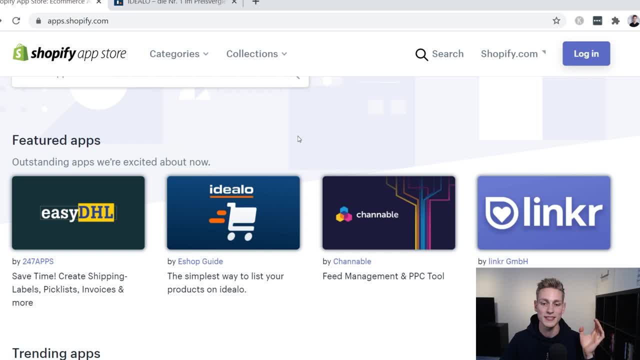 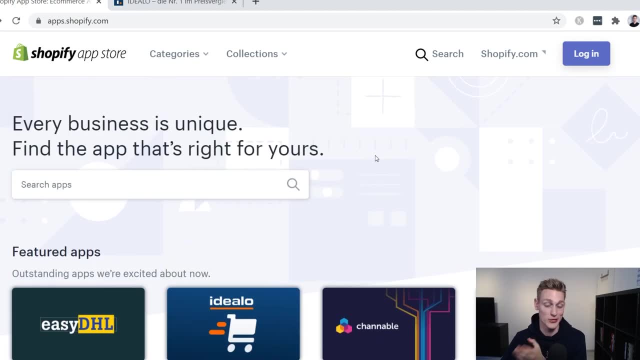 to show you an app that was built by the agency i'm currently working at. it is still pretty new and it was released about a month ago and, at least in my region, we are currently featured on the front page of the app store, which is also pretty cool, and, if you don't know, idealo is like a giant. 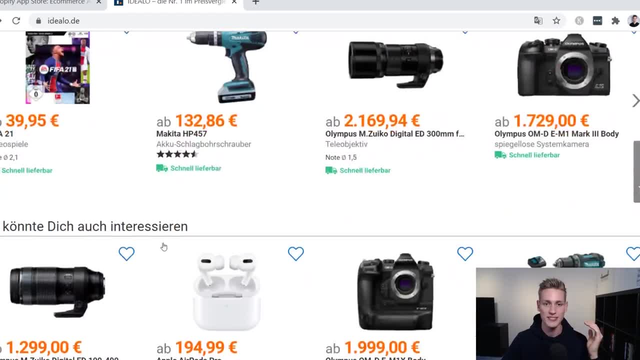 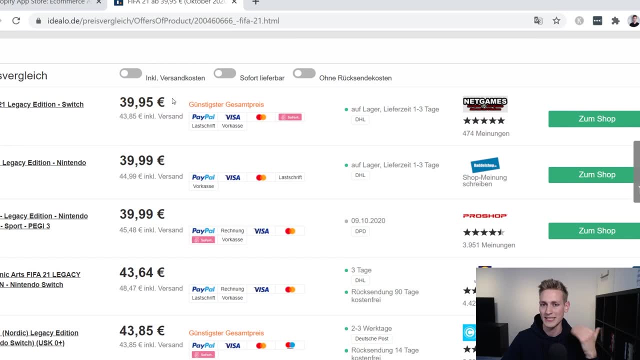 price comparison site here in germany with dozens of products, and if you click on one of them, you will find different listings from all the sellers offering this product, so that you can pick the best price or the best delivery conditions. and then you can pick the best delivery conditions. 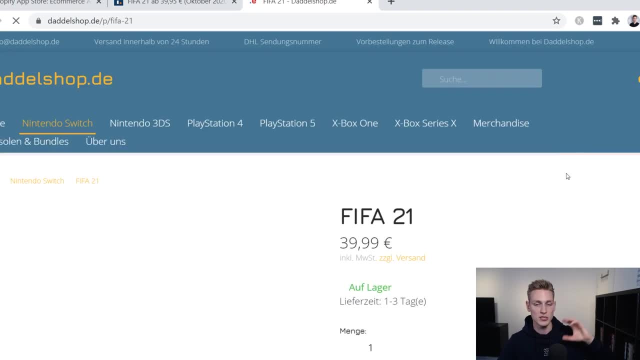 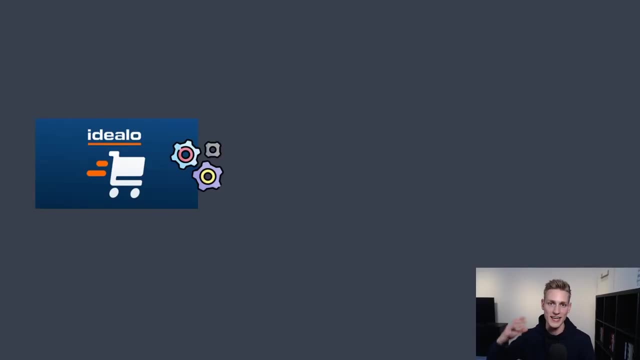 and if you click on one of these listings, you get redirected to the store itself so that you can buy the product, and that's an easy way for the seller to generate some extra traffic. and during the development, we got access to the idealo api where you can upload products. 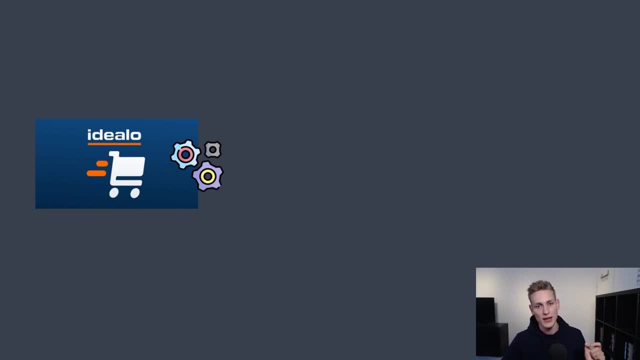 that you want to become listed on the platform, and our app now connects this api with the shopify admin api, where we retrieve all the product data and then we just pass it along to idealo so that you can get your products listed just by the click of a button and, of course, the 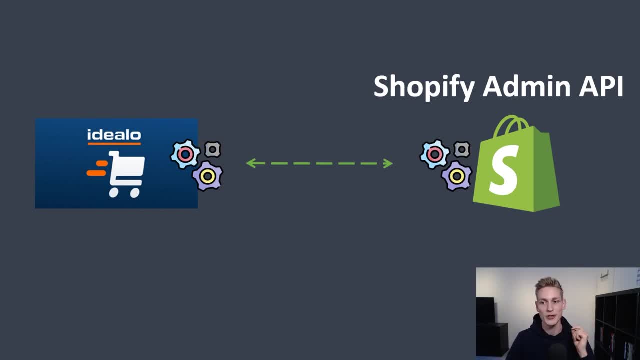 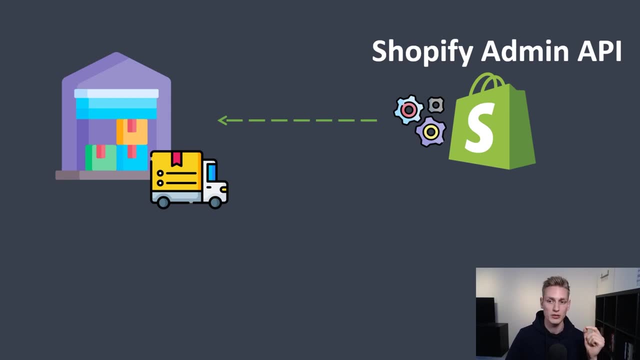 challenges are always hidden in the technical details, but that's the bird's eye view. another very common use case for the admin api is if you want to automate your order fulfillment, because then you can use the api to pass along the order details and your carrier can ship out the products. 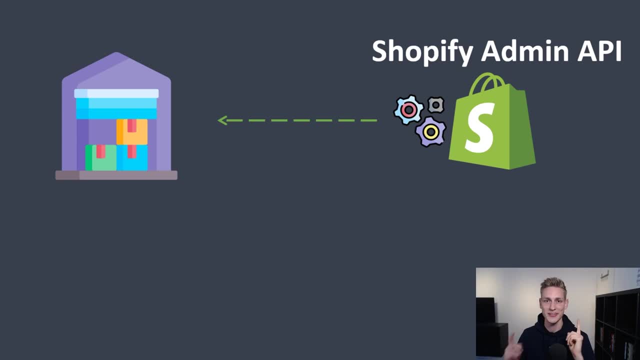 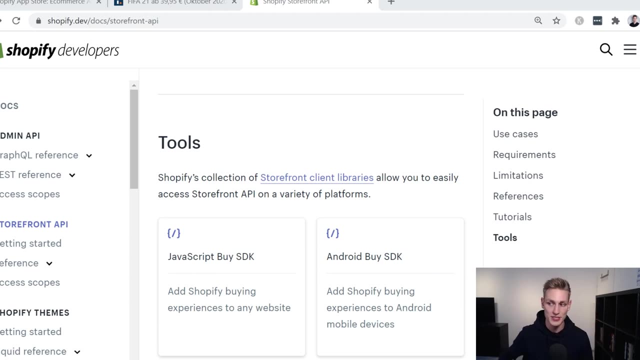 as per requirements, and now i just noticed that i had too much fun creating these presentations. all right, so now that we've seen a couple examples where one would leverage the admin api, let's also see some where you would need to use the storefront api, and i already told you that we can use the storefront api to build shopping experiences. 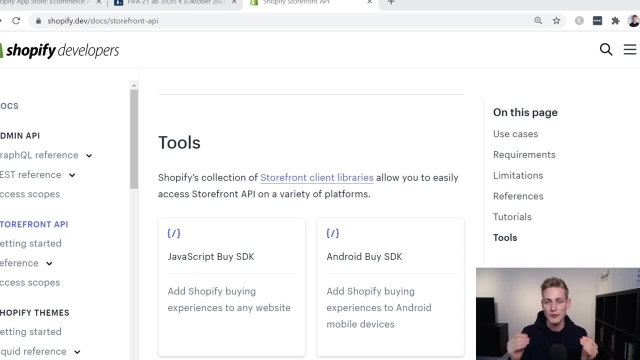 decoupled from our theme files. if you want to sell in different places than your online store- and these places could include different kind of apps like android apps, ios apps, maybe even react web apps- where you could then use shopify and integrate it as a shop system- 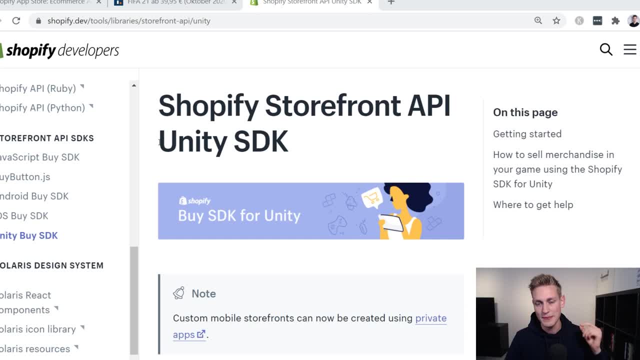 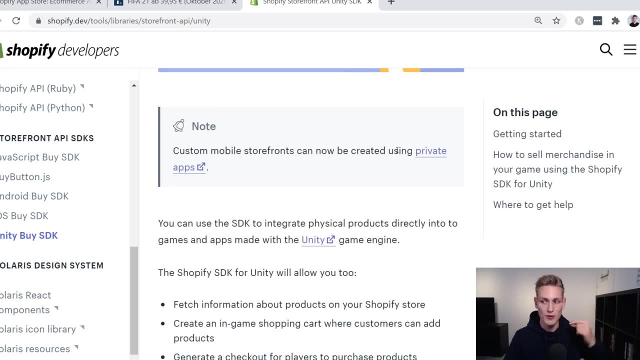 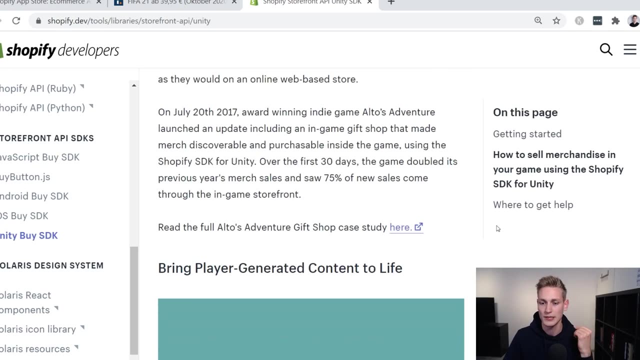 or what's also very exciting is: i don't know how much you are into gaming, but unity is a game development framework and actually you can connect or integrate your community with shopify and using the storefront api. you can then build experiences where the user could, let's say, make an in-game purchase for merch or if the, if the player generates some content in. 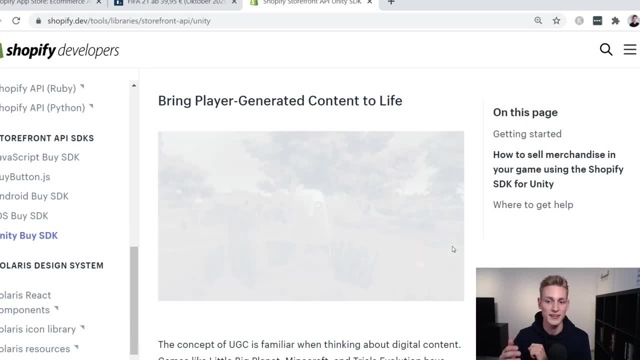 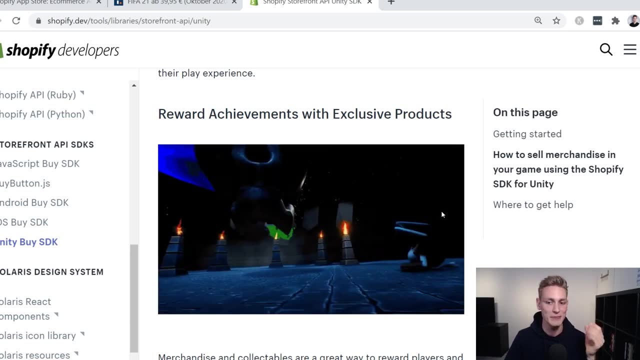 game. so, like in this example, someone is taking a screenshot of this guy and maybe you can connect a print on demand service to sell that image right away. or in this example where someone beats the final boss in an epic match and then he qualifies for the next purchase because he unlocks.